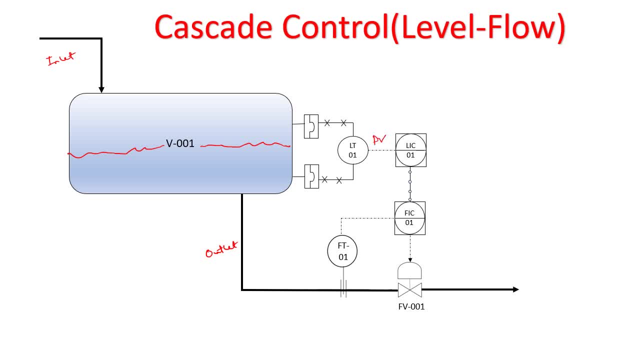 and this uh lic is getting set point from the operator and it generates basically mb. so in the ideal case what will happen is out in the normal- not ideal, i would say- in the normal bpcs case- what will happen is signal from this uh lic will directly go to. 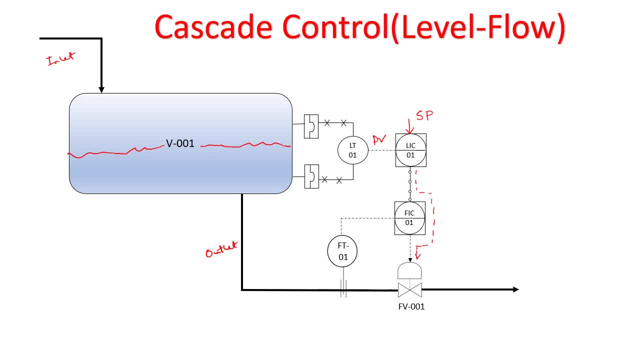 the valve, you and the control will be done. this will be mb. so whenever level increases or decreases, accordingly, pb changes and the mb will change and that will control this one. right, and that is how a simple process control works and that's what. what fine in most of the cases, right. 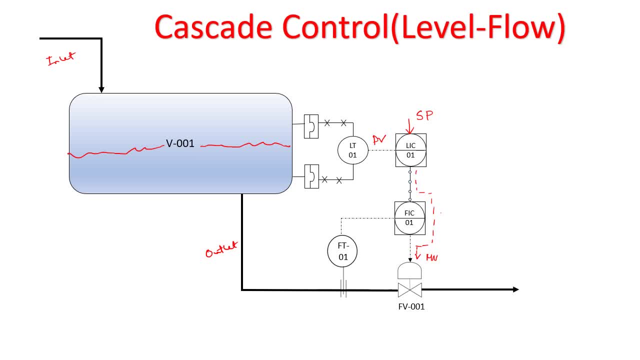 but what happens in this kind of a control if there is a large variation in the down stream process? so in the downstream there may be another valve right, there may be on a valve and there may be some other processes right. so suddenly, if there is something that caused this, 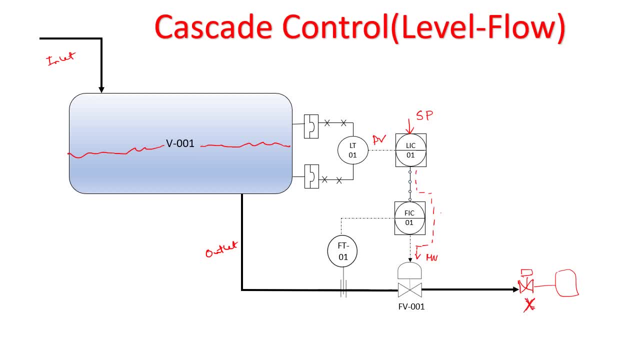 word to close, right, somebody closes this valve because of the downstream region, then what will happen? so the level, even if the controller is opening the valve or closing the valve, based on this level, due to the sudden closer of the valves, the outlet flow will get stopped and this will cause the level to increase. 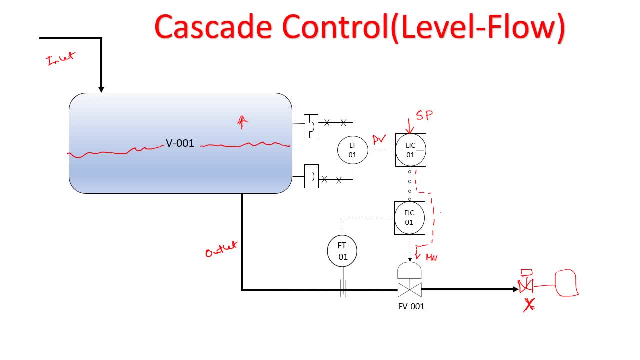 but this will take some time and by the time the level gets high and your level transmitter response and all the things happens. maybe the time is not sufficient to control the overspill right, because you see every time the process, there is a change in set point or there is some. 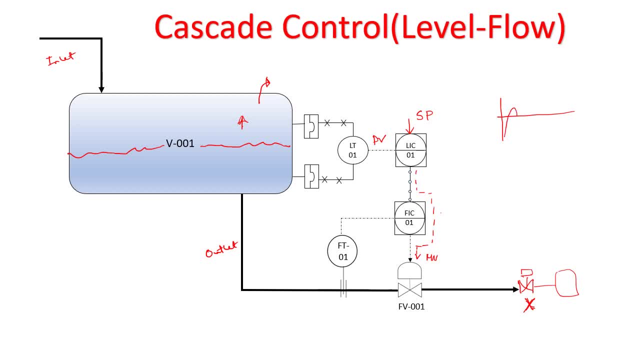 disturbance, the process does not immediately go to its set point. it goes through the cycle, right, and there is overshoot and undershoot also happens right. so this, so process stabilization takes time. so that's why, uh, the process design or process controllers, they thought that why not measure the thing that gets impacted first? 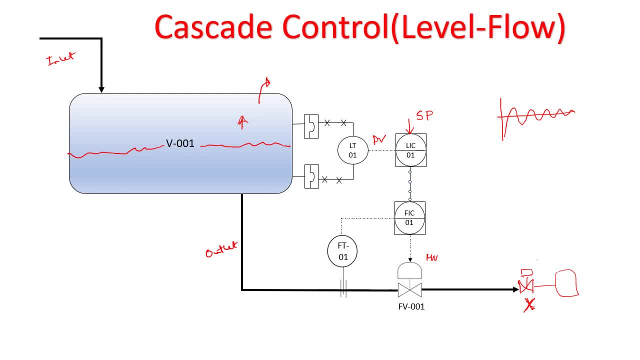 so here, here, in this particular example, when this valve gets closed, what get impacted first? what first senses that the valve is getting closed? it is the flow of this line. right, this flow of this line gets hit first and after that level, building up the level and then the level transmitter measuring. it will take some time. 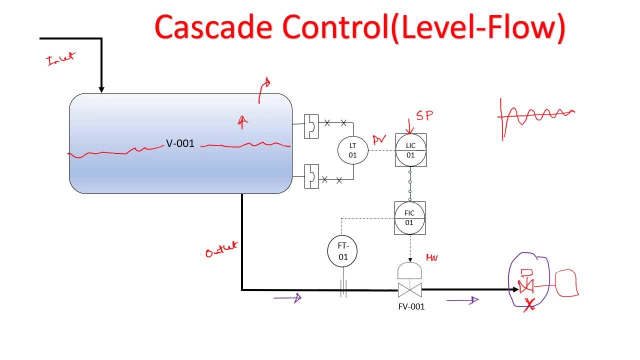 depending on how big the vessel is, how large the line is and everything. but for any cases, for any size of the vessel, for any size of the pipe, it is a flow that will always get impacted first, before the level. so that's why process designer thought: okay, let's install a flow meter here. this is a 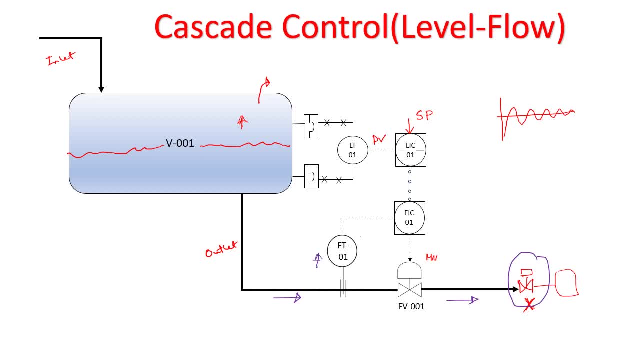 flow meter and sends the flow first. and let's have a flow controller and have a- well, have a closed loop with the flow itself, right? and instead of operator giving the set point to this fic, let's output of the lic right, which is the md, becomes a set point for this one. 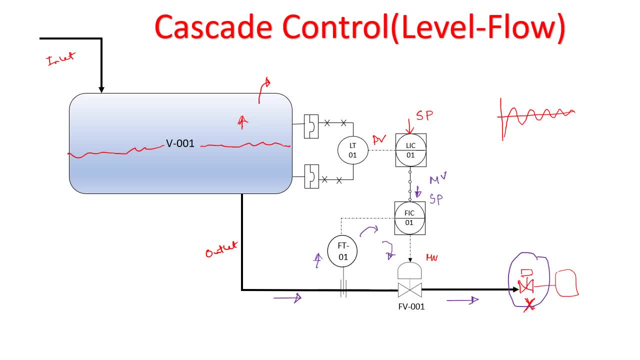 okay, so let's have much more clarity. okay, so, if we can denote them by two different numbers. so first of all, this first controller, our first, uh lt. its output: make it pv1. set point is sp1 and this output is mb1. okay, and it becomes the set point. so this become pv2. 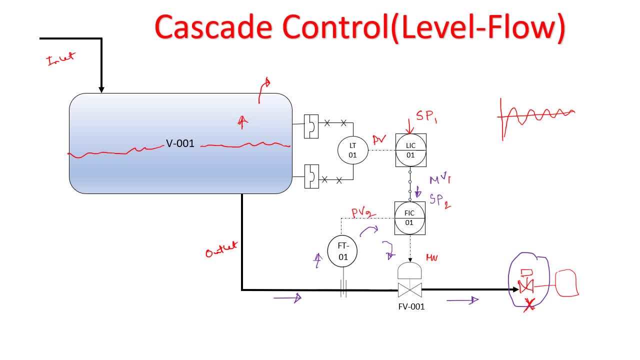 sorry, sp2, this becomes pv2 and this becomes mb2. okay, so output of the first controller, that is, mb1, becomes the set point of the second controller, right? so basically we are trying to maintain the level of the controller. so basically, we are trying to maintain the level of the controller. 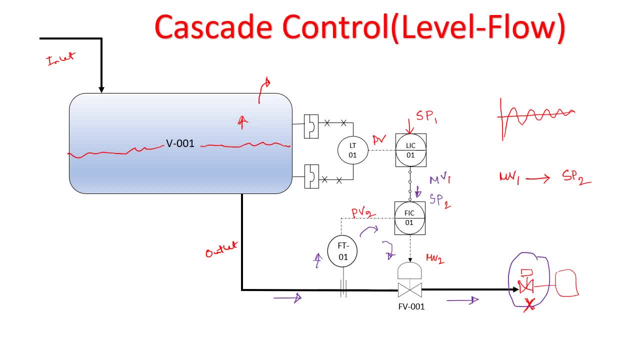 level, but we are doing it to the flow because flow is much more responsive to the downstream level. but we are doing it to the flow because flow is much more responsive to the downstream disturbances. if there is no disturbance, flow will remain the same and uh, and there will not be much. 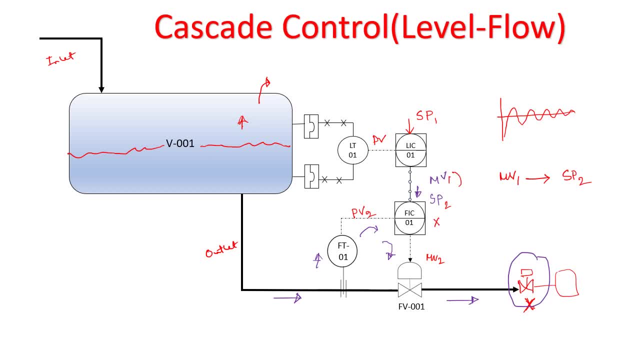 of a action this fic will do. it will simply pass on this mb2, sp2, right, okay, and this is the way it is depicted in the pnad also, you see there is a controller here. so this is the first controller here and this is the second controller here, or second control loop. 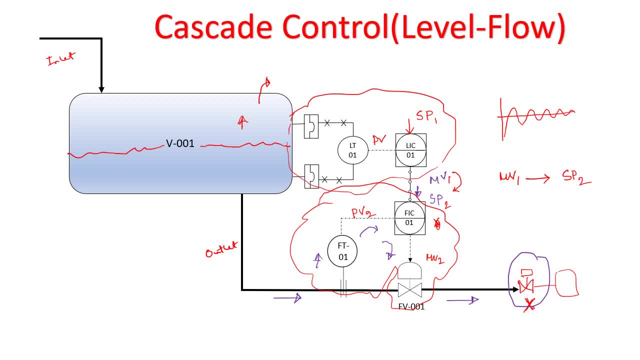 here and between them, the link is a software link, because this communication, this line- if you go back to our earlier lectures where we have discussed about what is the meaning of the different links, these particular links, provides you a description of a software link. so this is basically a software link. let's erase them, everything, so that 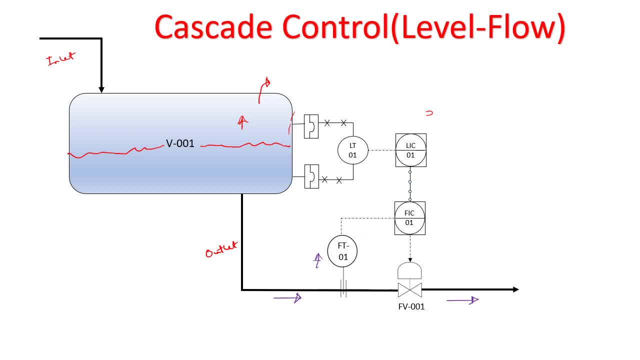 becomes easy to understand. okay, okay, okay here, okay, so controller, and this is the sleep control and this is the software link I was talking about. and this signals is the electrical signals, so you, if you are still confused about the no symbols of different lines, so this is the electrical and this is the software signal. and 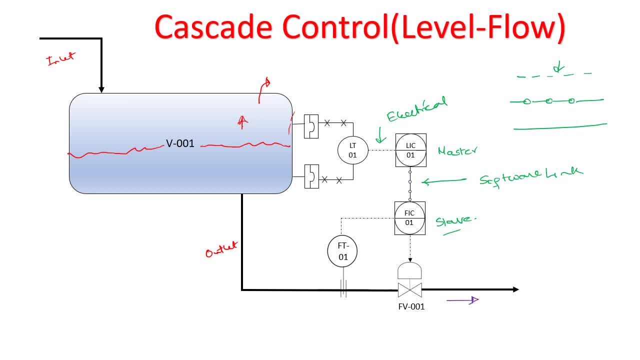 normal line means it is a process line. so if you are still confused, you should go back to earlier lectures and see what is the significance of the different line. this particular symbol is of an orifice and this is a global, and this particular LT is a diaphragm seal LT. these are the this. 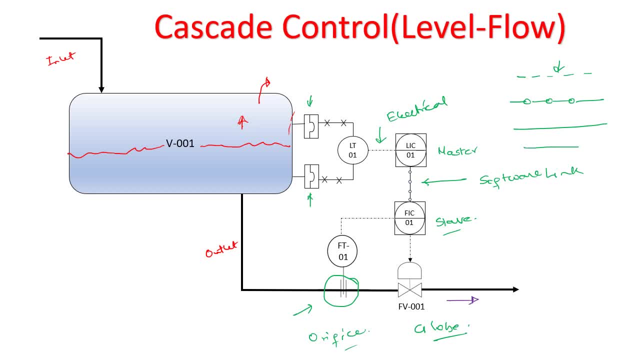 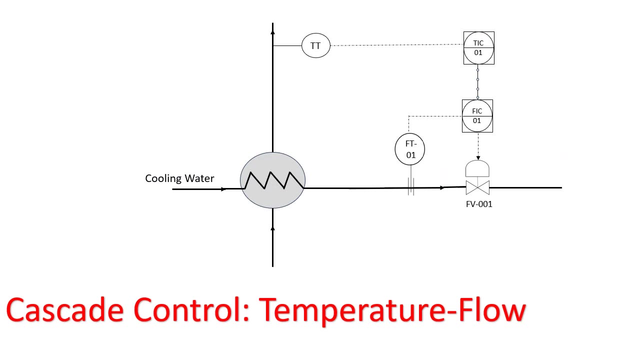 signifies the diaphragm and this particular line signifies the capillary. okay, so hope this is clear to you. now we'll be taking another loop. so this loop is our temperature Loop. for this also we earlier we have discussed about um, the basic process control Loop. so here there is a medium or there is a. 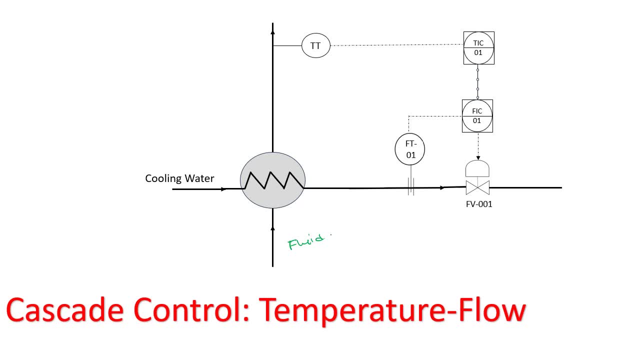 fluid which is getting cooled. right. it is getting cold. for example, take this as a sub hydrocarbon: okay, and it is getting cooled through a heat exchanger by the cooling water. now the temperature of the outlet of the hydrocarbon is to be maintained because of the downstream process, how the 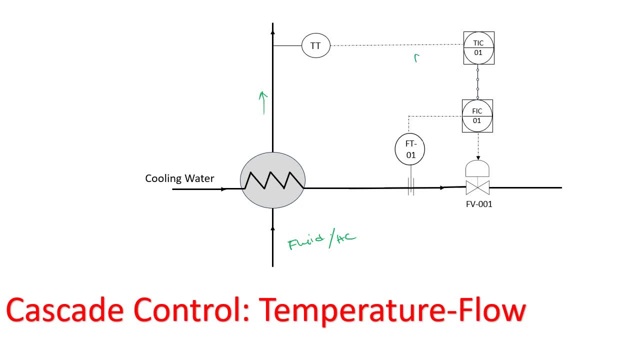 temperature is sense. temperature is sense through a TT. TT gives the signal as the form of PV to the temperature indicator controller. in the case of the basic process control system, there is a set point here and this output actually goes directly to the valve. right. there is. this was not there. this was not there. 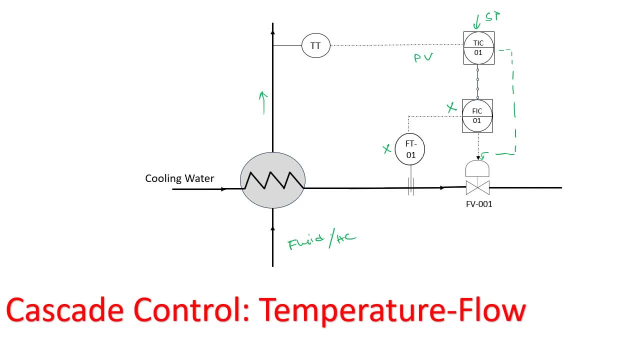 and simply, when the temperature increases or decreases, depending on that, this valve opens and closes and this is how the temperature is maintained. but what happens? if there is some restriction here or some some valve here that gets closed or the line gets choked or something happens right, then the flow, this cooling water flow, gets stopped or gets restricted right, and this will 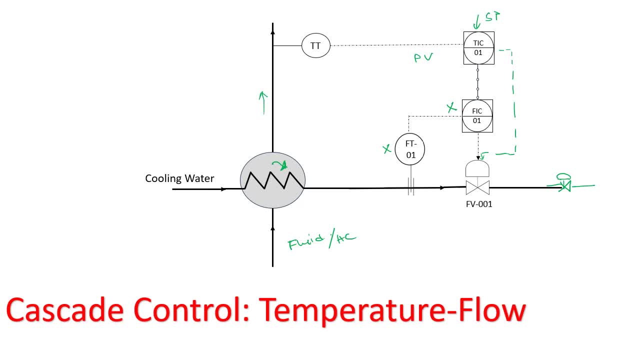 this will increase the temperature of the fluid, but it will take some time. maybe it can take 10 minutes of time to actually uh, due to the loss of the cooling water, this fluid gets heated and after 10 minutes the temperature sensor understands it and sustain the signal to the 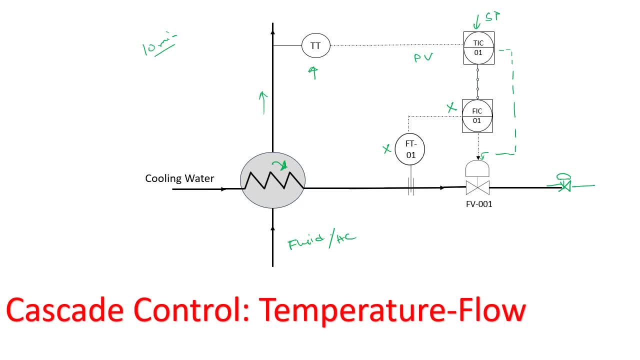 TIC, and then the action goes here, right, so it may be so late. in that situation, what is the parameter that gets impacted first? it is the flow. again, your flow is gets impacted first and much before your temperature, right. so that is why the process designer what they do, they take this flow as a secondary loop to this master loop. so here it is.